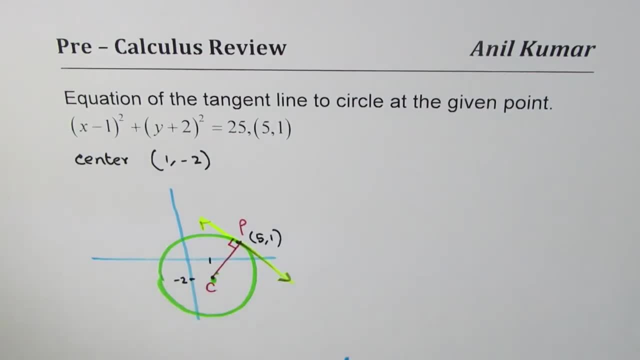 to find the equation of the tangent line. so I hope with this you understand the whole concept right. so once that is clear, let's begin how to find equation of tangent line. so first thing is we identify what Center is. Center is at 1 minus 2 and the point P given to us is 5: 1. so using Center C and the point P, we 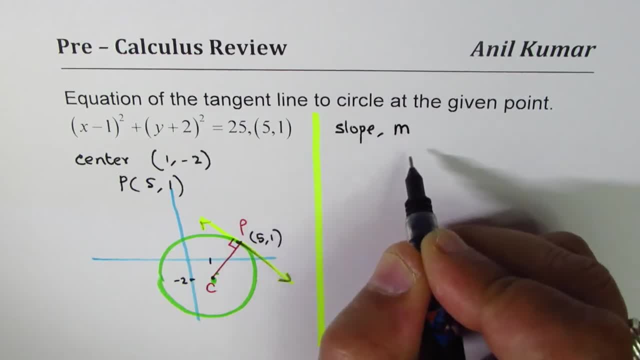 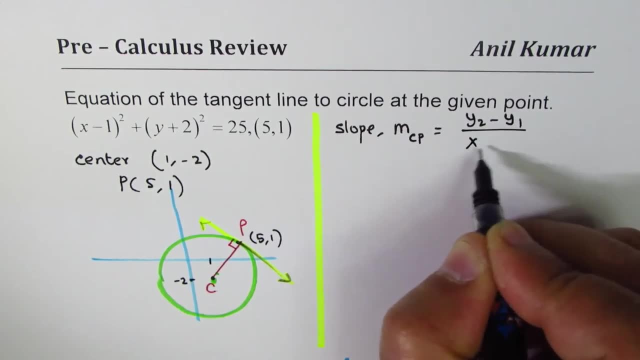 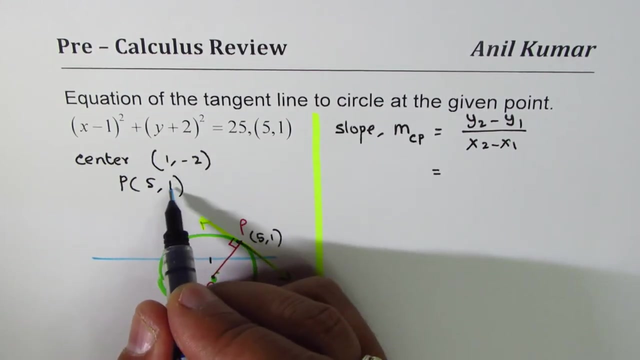 can find slope. let's call this MCP. slope of MCP will be. the formula is y 2 minus y 1, divided by x 2 minus x 1, that gives me 1. so these are the two points, right. so 1 minus 1 minus minus 2, divided by 5 minus 1, right. 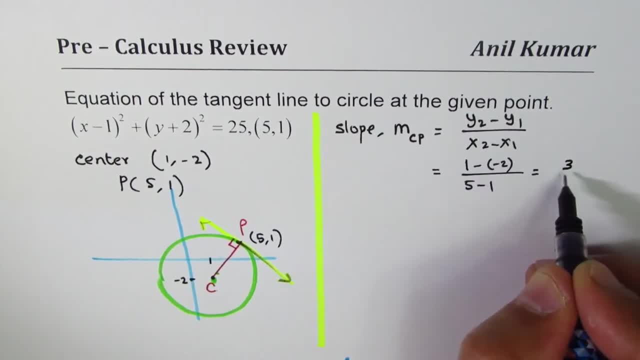 5 minus 1, that makes it 3 and this is 4. now let the slope of tangent line be empty, right, so empty now, since this is perpendicular, is going to be negative, reciprocal, right, so negative. 4 over 3 doesn't make sense to you, correct? so 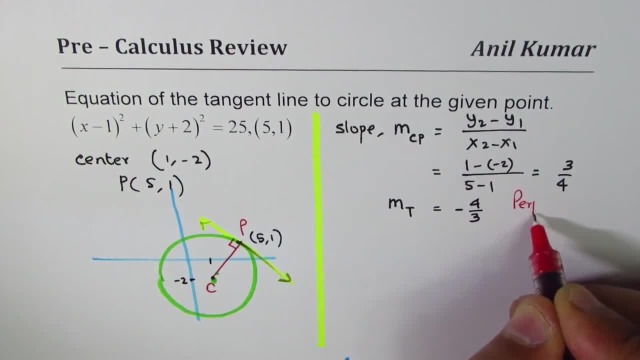 since it is perpendicular, right correct. now, if the slope of the line is minus 4 over 3, then the equation could be: Y equals to minus 4 over 3X plus P. to express this slope of the line, we wouldfounded x plus P. so is the concrete line angle of xcombining x and subscribe. and now if this slope of the line isционallyeee? system, so that the search below, if you choose to find this equation, the sin over 3, sir, compare to guess: y equals to minus four, Y equals to minus 4, which is person and can be that particular to find out where is constant right. and now a whole lot of assuntoa mas. 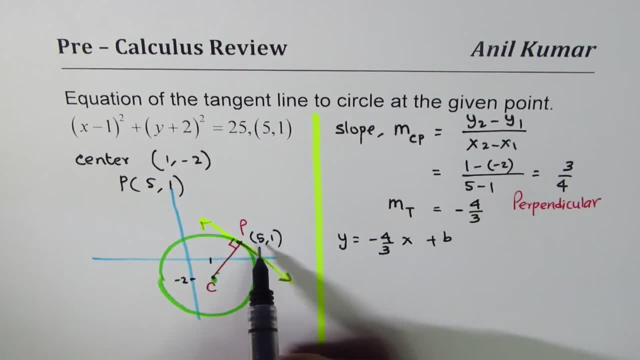 the value of B. we can use the point 5, 1.. X value is 5, Y is 1.. We get 1 equals to minus 4 over 3 times 5 plus B. Taking it to the right side, this becomes 20 over 3,. 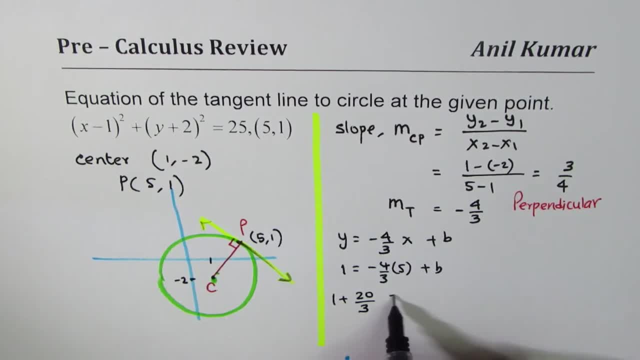 right. So we get 1 plus 20 over 3 equals to B. So if you take common denominator right, 3.. So you get 3 plus 20 equals to B, which is 23 over 3.. Is that okay? So once. 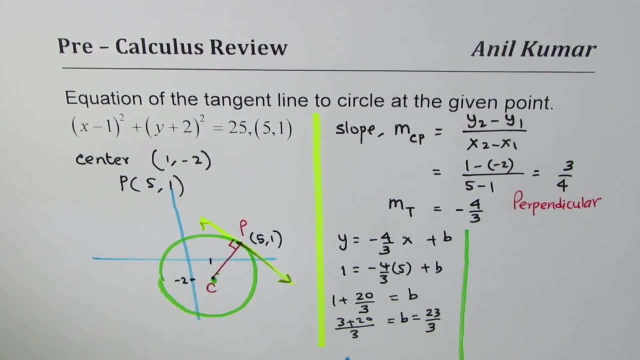 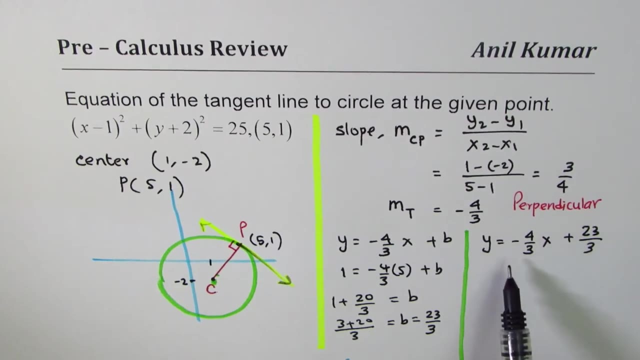 we know the value of B, we can easily write down the equation of the tangent line. Substituting this: here we get: Y equals to minus 4 over 3, X plus 23 over 3, right, If the question is to write this in standard form, you should know that technique also. We just 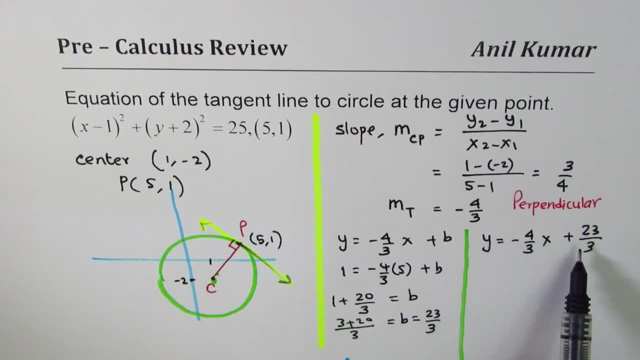 need to bring all the terms. on one side, We can multiply by 3.. So we get 3Y equals to minus 4X plus 23.. Bringing them to the left side, we want to keep coefficient of X positive, right, So we get 4X plus 3Y minus 23 equals to 0, right, So you could write. 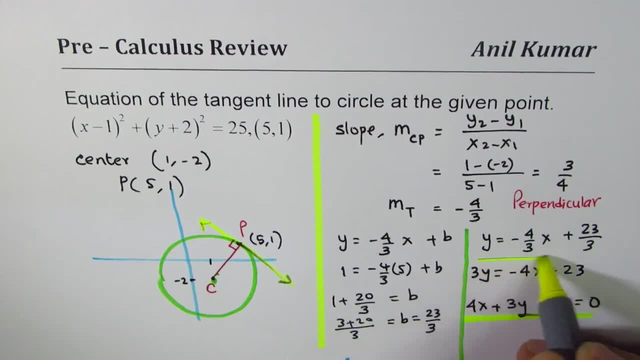 the answer in standard form or in slope intersection. But we don't need to write the answer in constant form if it is not given or specified in the equation. But I hope with this you understand the process of finding equation of tangent line to circle at a given point. I'm Manil Kumar and I hope that helps You can put. 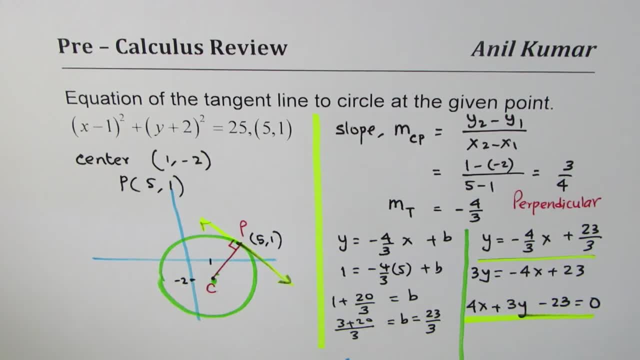 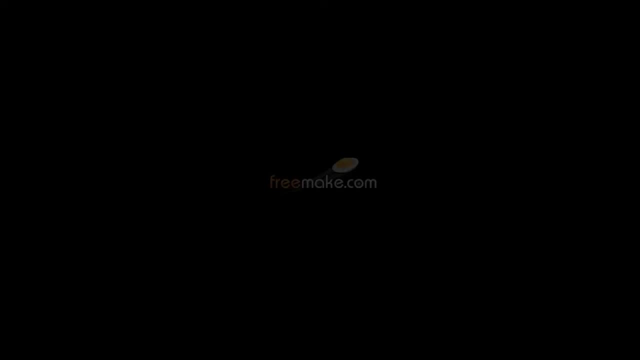 some likes. if you like my video, Share my videos with your friends and don't forget to write comments. Thank you and all the best. Thank you. 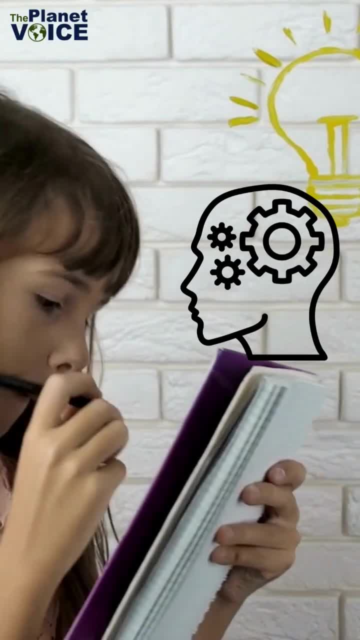 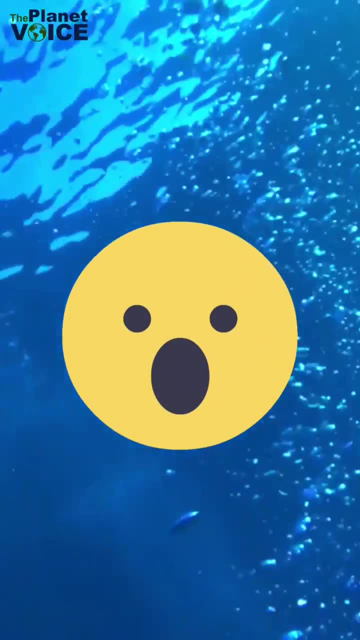 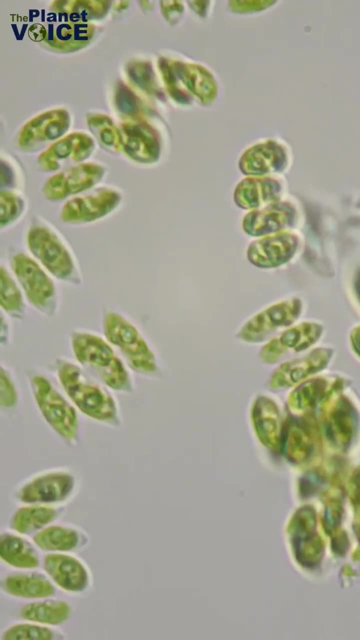 Whenever we hear the word oxygen, what is the first thing that comes to your mind? Trees, right, But did you know that the oceans produce more than 50% of the oxygen on our planet? All thanks to a little organism known as phytoplankton. All ocean ecosystems contain 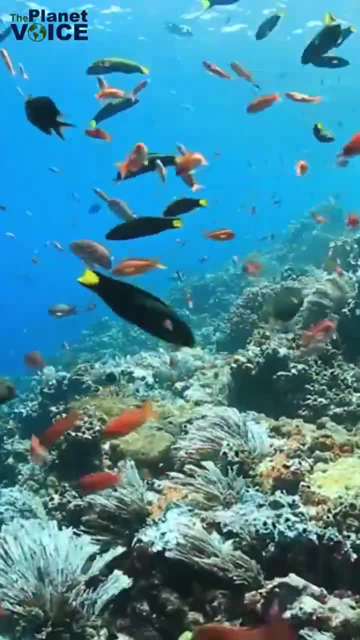 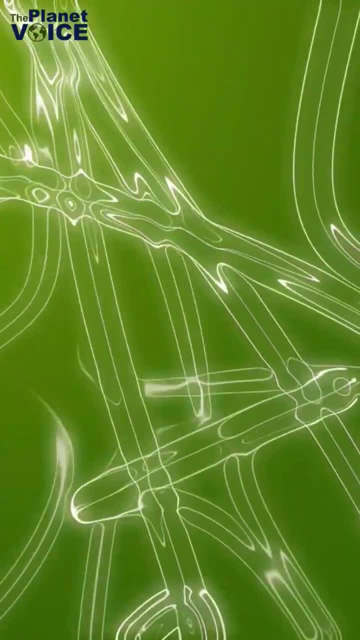 marine phytoplankton, which is essential to preserving the harmony and health of the ocean and its intricate food webs. Photosynthesis is the process through which phytoplankton grows. Oxygen is released into the water by phytoplankton during the process of photosynthesis. 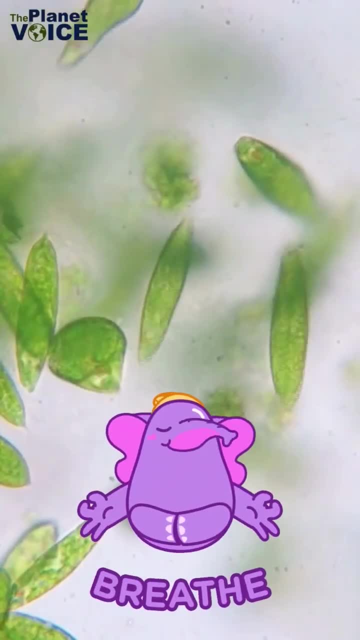 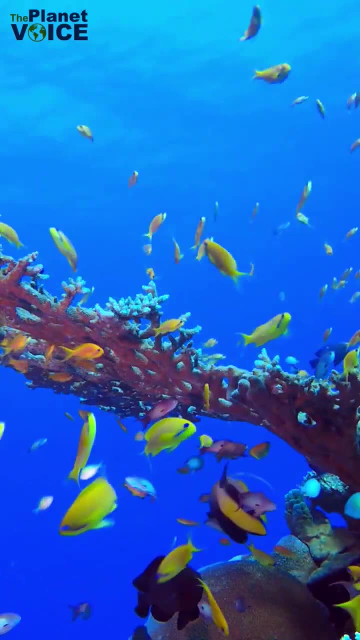 Since the oceans cover 71% of the planet, phytoplankton are in charge of producing more than 50% of the oxygen that humans breathe. Phytoplankton is ultimately responsible for producing all the food in the ocean. Phytoplankton play a significant role in the climate system.